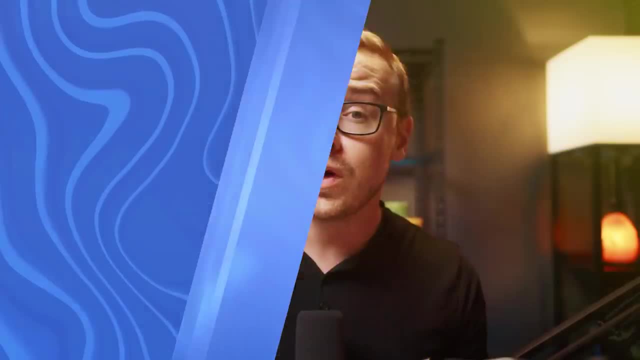 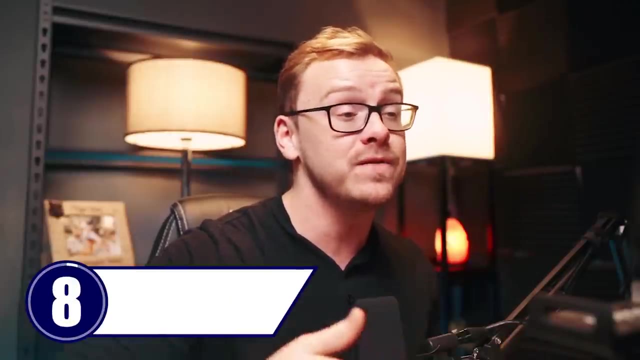 that milestone than if you've got a useless degree. Now the first one on the list is going to be a business related degree, And this one combines business skills with technology skills, with an emphasis on data. You see, data is more valuable than oil or gold And companies. 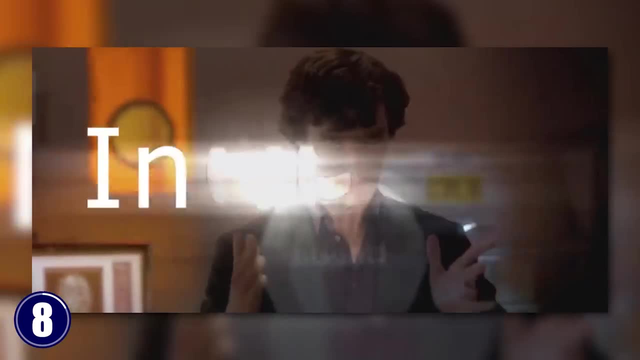 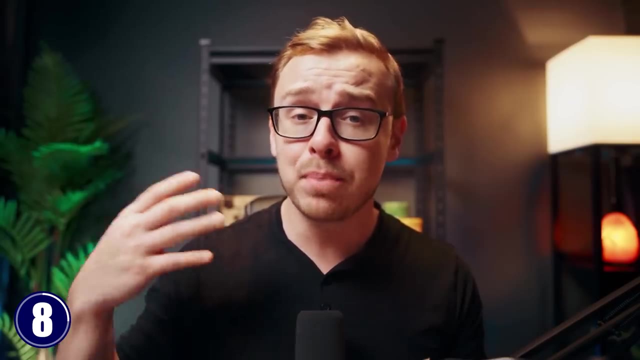 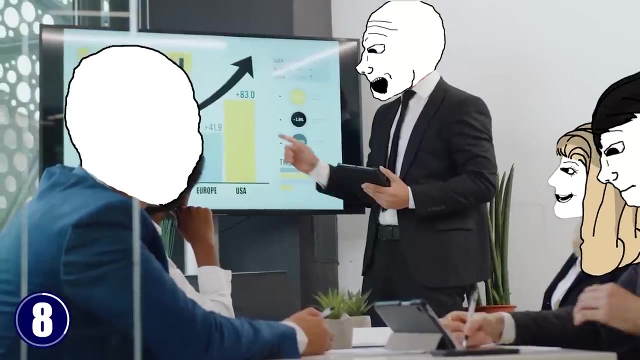 need people who are good at organizing and making sense of all the data that they get, And that's where you come in if you get a management information systems degree. So this degree is basically a perfect combination of technology skills and business skills, And just about every business in every single industry out there needs people that have 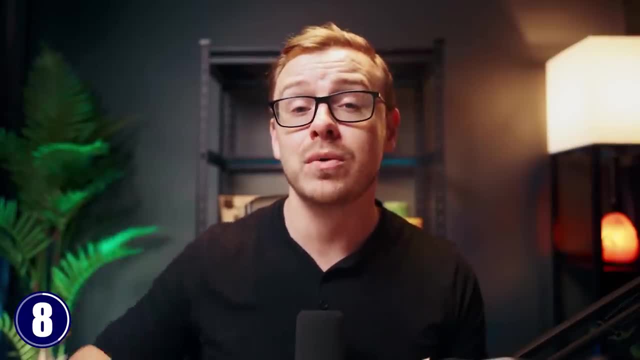 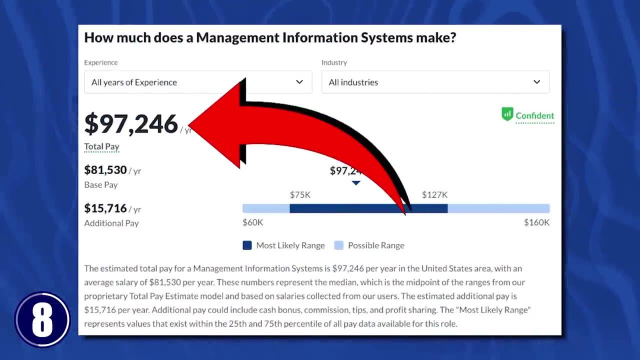 these skill sets And that's why you see insanely good numbers when you look at this degree. So, for instance, when you type in management information systems on Glassdoor, you're going to see they look like this. And when you look on BLS, it's growing at 16% over the next 10 years. So yeah, 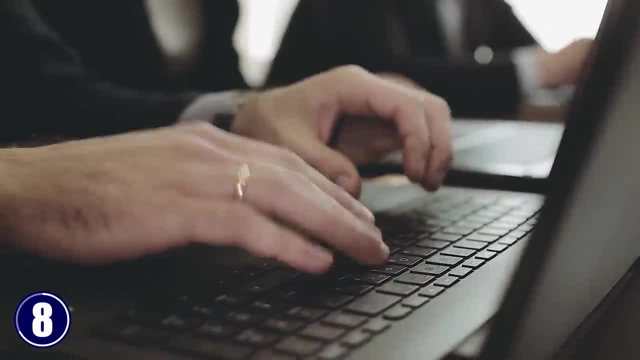 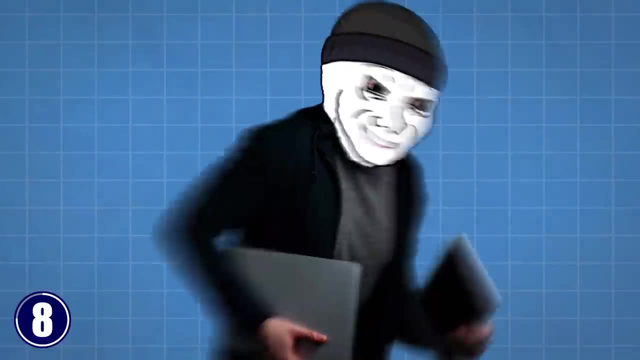 there is a lot of positives to getting this degree. I will say that the way that companies collect data is extremely sketchy. They basically stole our data without our permission and they pretty much got clean away with it, And the reason they're able to do that is because a lot of the 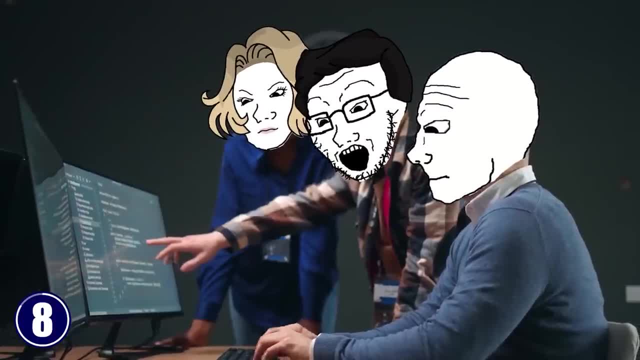 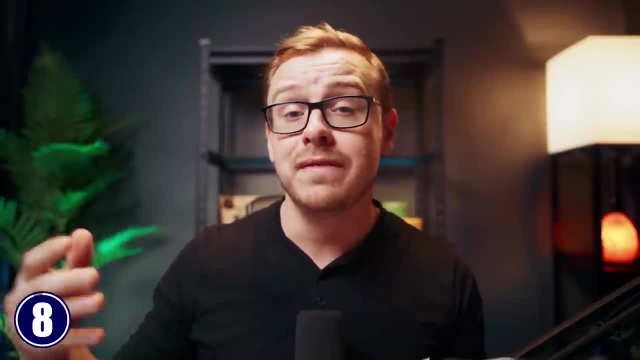 big technology companies are basically proxies for the government to do what they want, And hopefully that doesn't involve them using that data to control people against their will. And, by the way, if you find this content to be valuable, go ahead and subscribe to our channel. 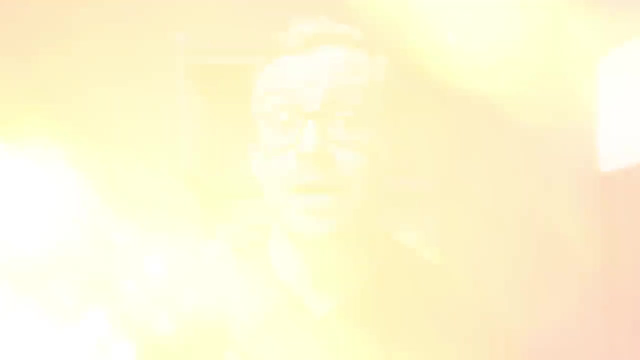 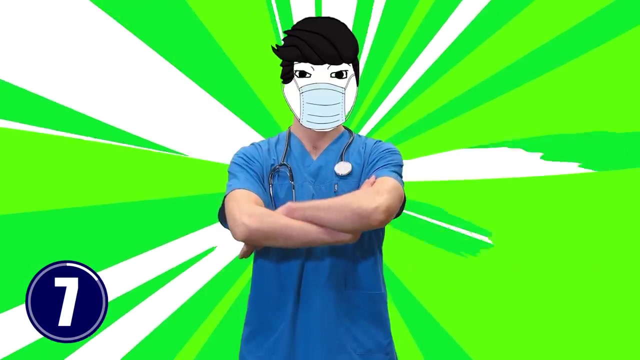 Gently tap that like button and the algorithm will serve you more of it. Now, the next one on the list is going to be a health related bachelor's degree, And this one's kind of like being a superhero, except instead of wearing a cape, you're going to be wearing scrubs and a stethoscope. So 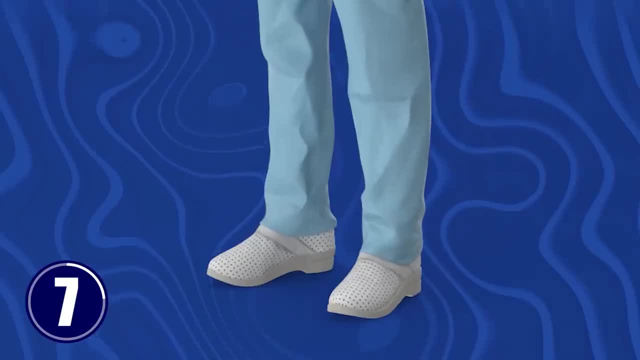 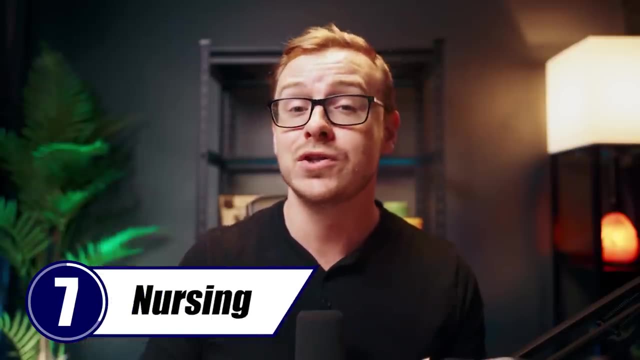 you should get ready to save lives and be on your feet all day, So make sure to buy some really good, high quality shoes- And of course I'm talking about nursing, No, but seriously, if you want to buy a good pair of shoes, just find one of your friends who's a nurse, and I can almost guarantee. 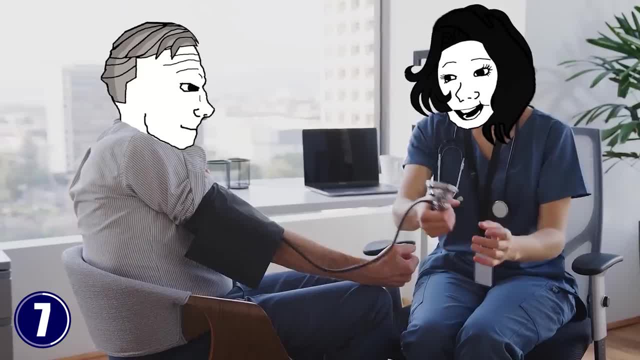 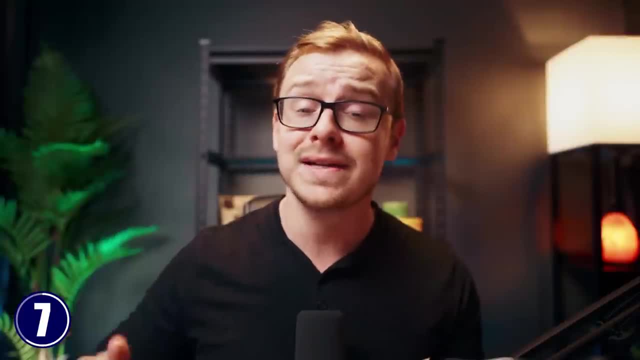 you. they're going to tell you the best one Now. nurses are basically the foot soldiers of the healthcare industry. right, They're like on the front line in the war against death and injury, And I know that sounds kind of morbid, but literally nurses are like the backbone. of the healthcare system Now, entry level nursing jobs. you're going to make about $69,000 a year, but I can almost guarantee you if you specialize you can make way more than that. I know nurses who make several hundred thousand dollars a year and it's growing at about 6% over the next 10. 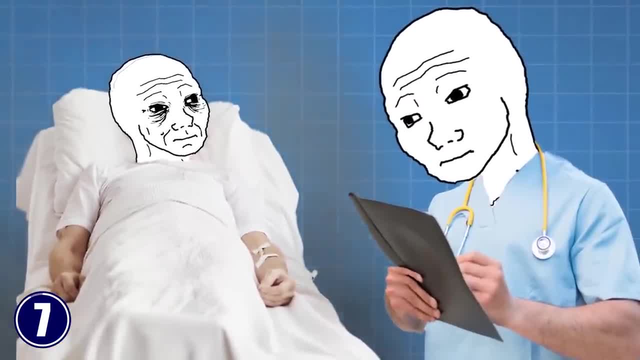 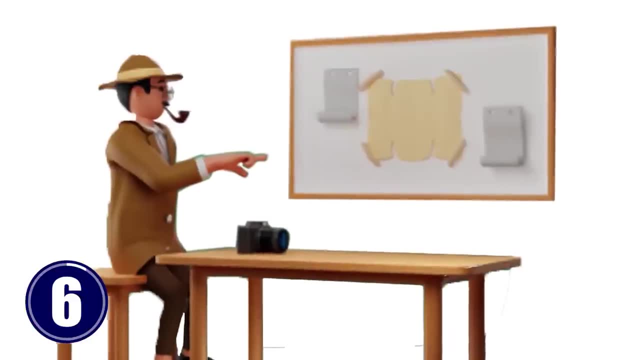 years. So this one is great for people who love helping other people, And it's not so good for people who get queasy at the sight of blood. Now the next one is going to be for my math nerds out there, And it's kind of like being a detective that solves mysteries with numbers instead of 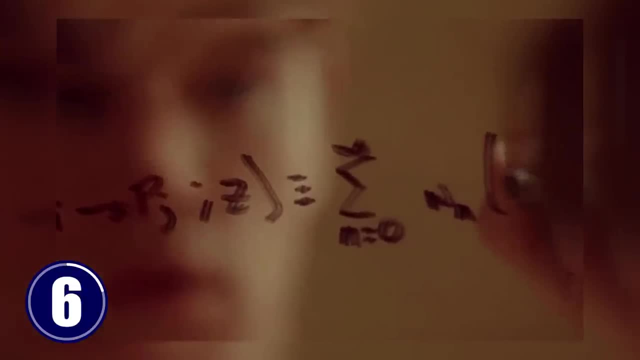 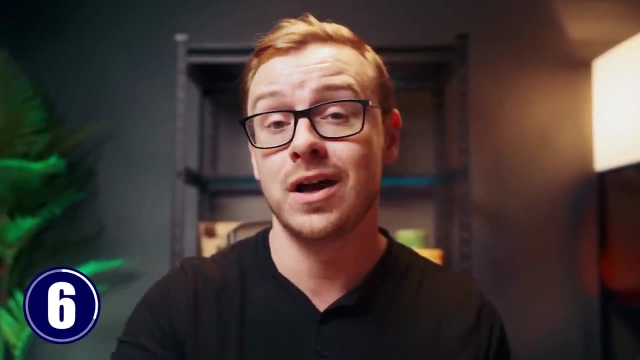 clues, So you'll need to be good at math and have a sharp eye for detail, And the degree I'm talking about is going to be statistics. So remember when I was talking about data and how valuable it is to companies. Well, one of the main ways that companies get actionable insights from that data 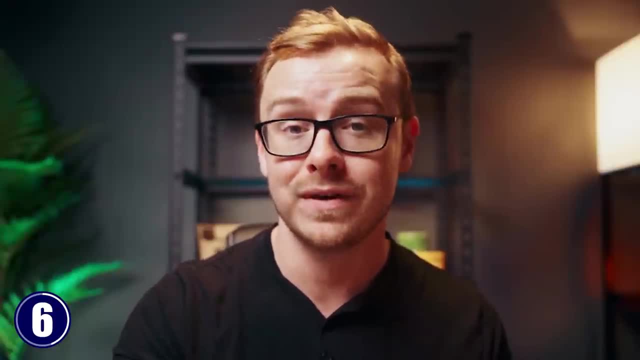 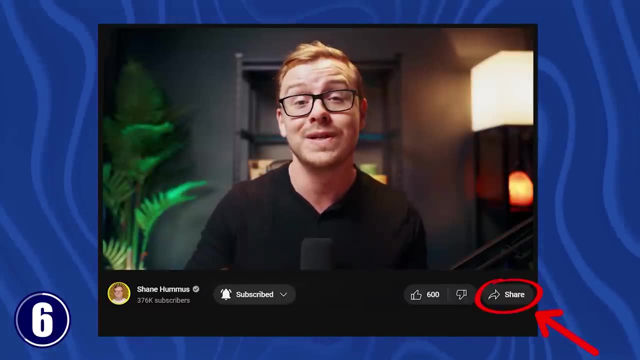 is they hire people who are good at statistics to make sense of it. Now, speaking of statistics, I'm going to give you a better chance of getting a girlfriend if you share this video with a friend or family member who needs to see it. It's science, I mean. just about anything passes for science. 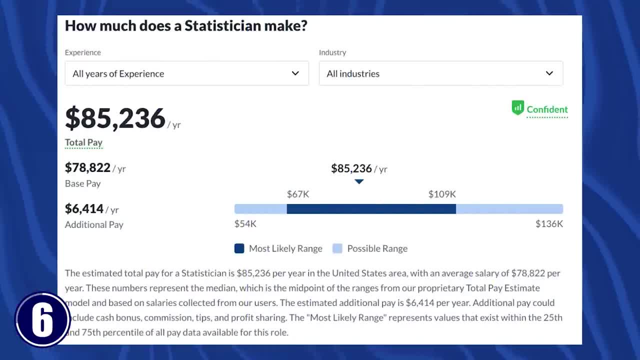 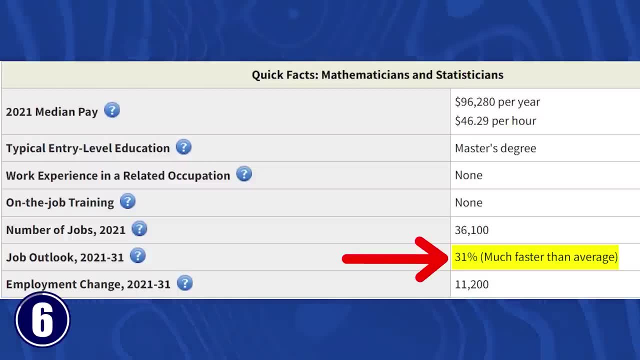 these days. So hey, it could be true. Now, all joking aside, statisticians- really hard to say that word- make about $85,000 a year, and it's growing at 31% over the next 10 years. So this: 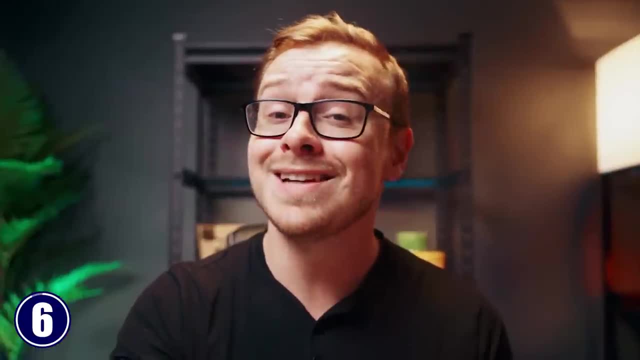 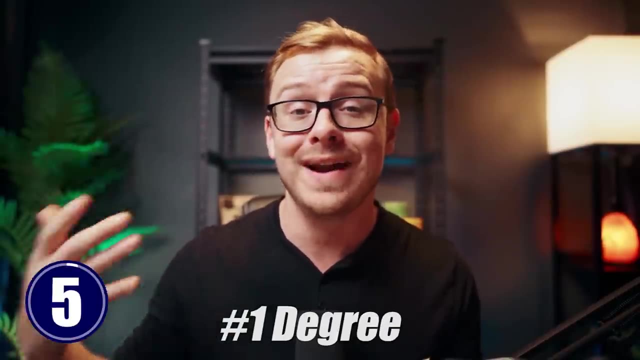 one is great for people who love math, logic and puzzles, And it's not so good for people who find numbers to be more confusing than words. Now, the next one on the list came in as my number one- over 900 different degrees on my college degree ranker, So this one has insanely good statistics. 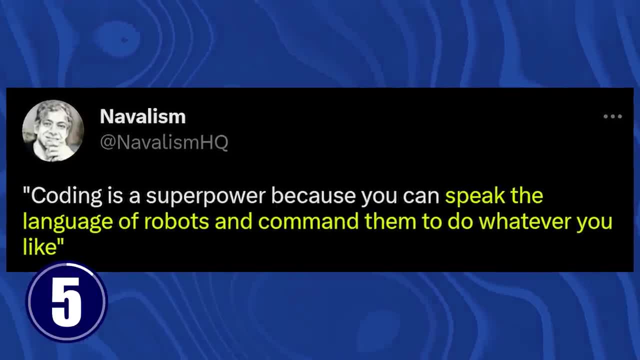 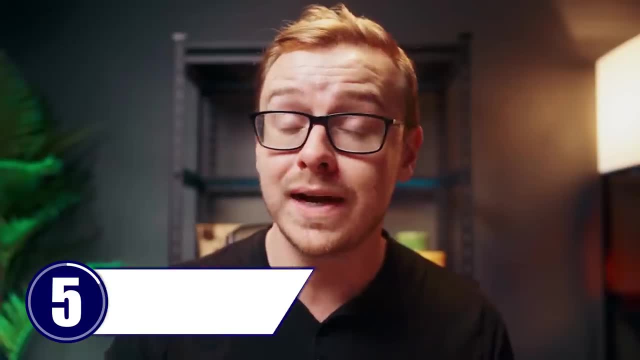 And it's basically like speaking the language of robots and being able to command them what to do, And you're probably able to guess which one it is. Yes, it is computer science, And computer science will probably lead you to a job as a software developer, And, if you haven't noticed, 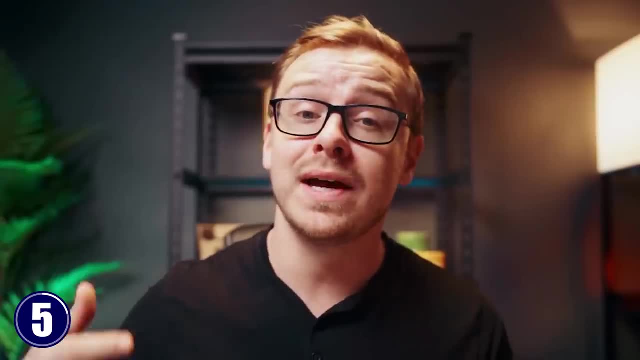 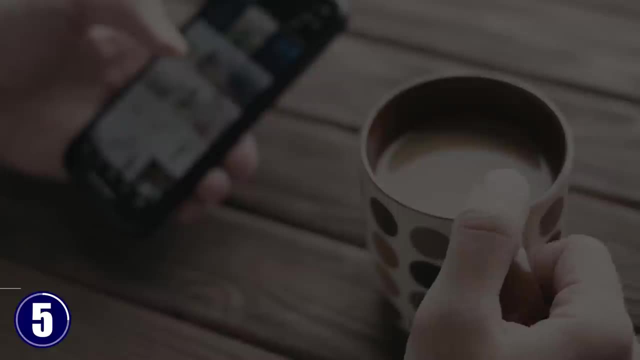 this world basically runs on technology, And computer scientists are the ones who are making sure that it's running properly. Now I'll be honest with you. I think technology has gone a little bit too far. There's a lot of studies that have shown that depression and anxiety and 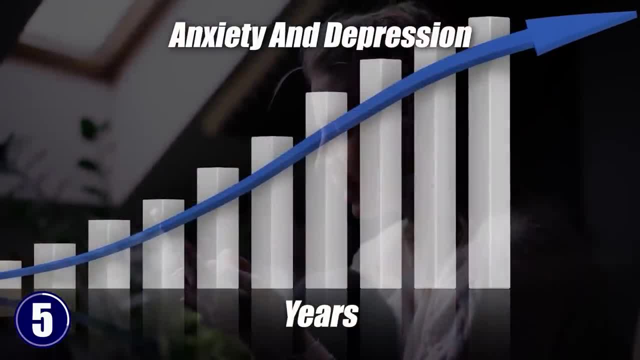 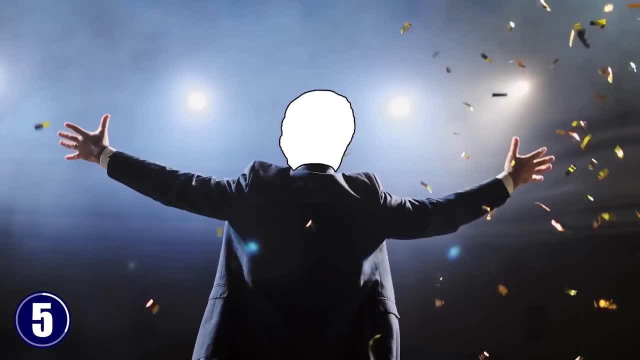 other mental disorders have actually gone up since the onset of social media, So I really do think that you should limit your exposure to technology. And I think the most important thing, this is probably going to be the difference between the people who are successful and not successful. 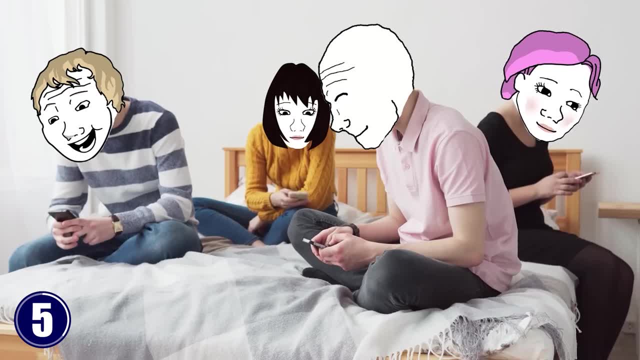 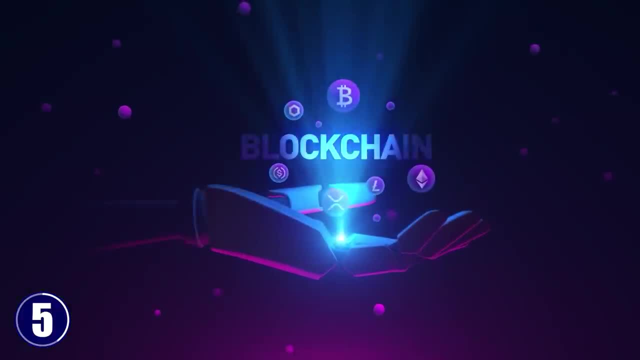 is your ability to use technology and not let technology use you. But there's a lot of really cool things coming out in technology. For instance, I'm a huge fan of cryptocurrency and the blockchain, but it can also be used for bad. So, for instance, I'm a huge fan of cryptocurrency and the blockchain. 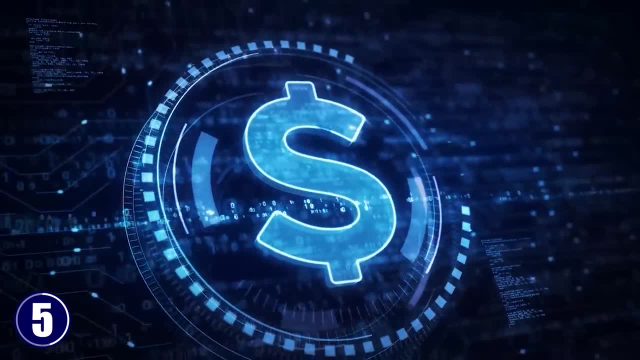 but it can also be used for bad. So, for instance, I'm a huge fan of cryptocurrency and the blockchain, but it can also be used for bad. So, for instance, I'm a huge fan of cryptocurrency and the blockchain. governments now are saying that they are going to try to create their own versions of digital 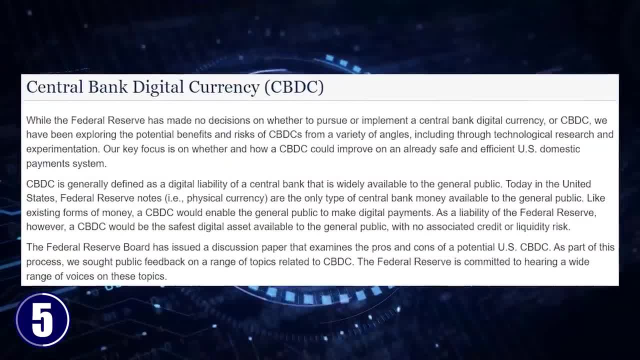 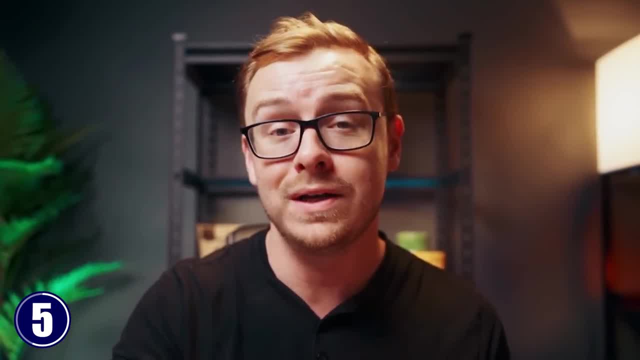 currency known as CBDCs, which is Central Bank Digital Currencies, And that is absolutely terrifying because they will be able to control what you're allowed to spend your money on right. So if they think you've been a bad boy, you might not be able to buy a car or get transportation. 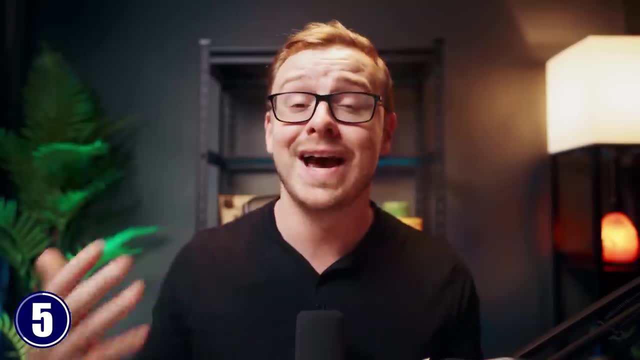 or they might limit the amount of meat you can eat, right? It's really actually kind of terrifying. And they literally say that you're going to own nothing and be happy. So what I mean by this is technology can be used to control what you're allowed to spend your money on. So what I mean by this is: 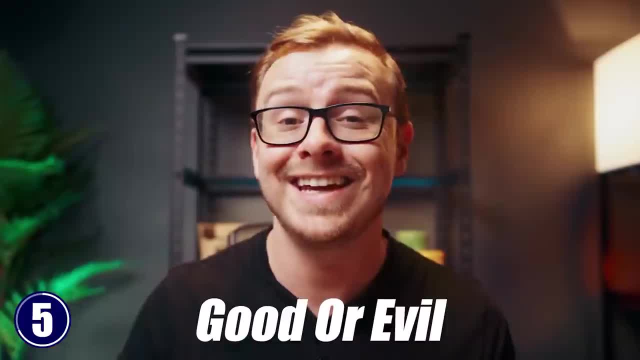 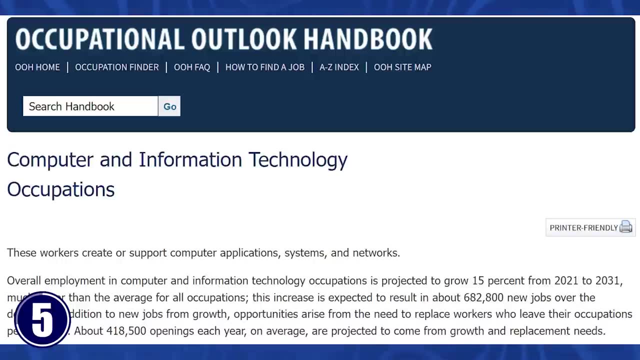 technology can be used for good or evil. It's a tool just like anything else. Now, as a computer scientist, you would be expected to make about $115,000 a year, And these types of careers are growing at about 15% over the next 10 years. Now, speaking of technology, there are a bunch. 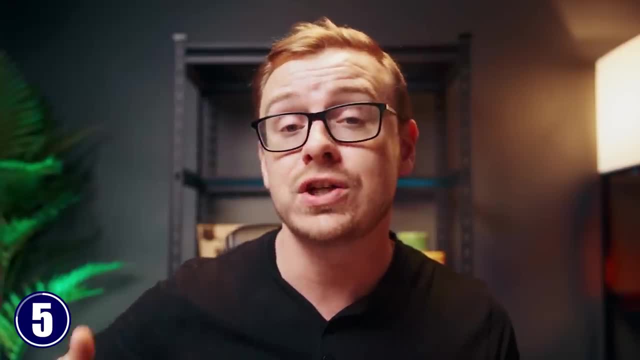 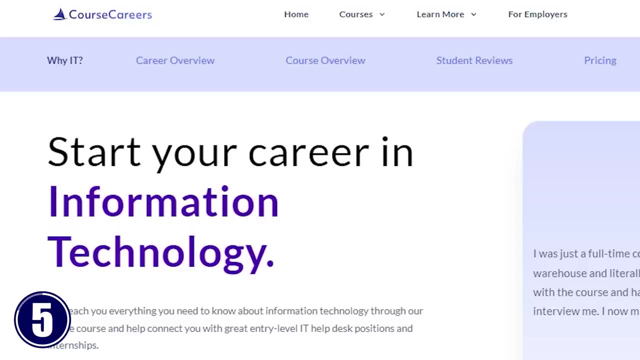 of different great technology careers out there that you don't actually have to get college degrees in order to get into- And the sponsor of this video is going to be Course Careers- and they help people get into IT related careers in a very short period of time. So, for instance, I've 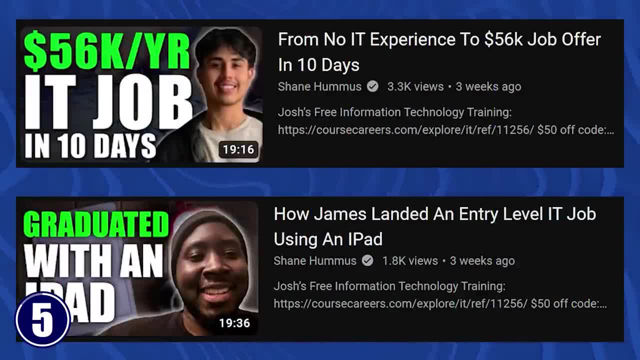 interviewed people on this channel and they've said that they're interested in learning about how to get into IT careers in less than a month. So definitely check them out. They have a free training which I'll put down in the description below, where they'll kind of go over how you can. 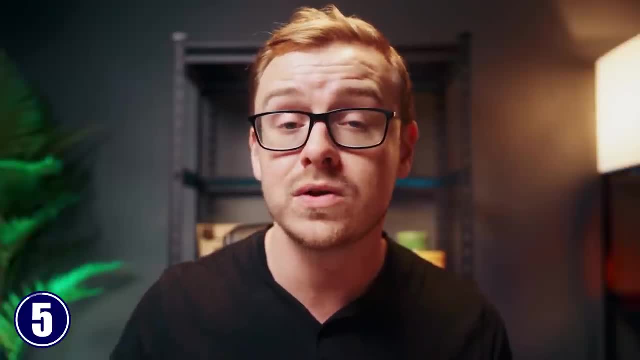 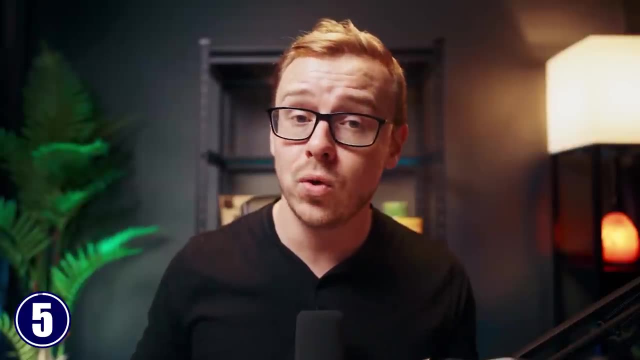 get into an IT career. they'll explain to you how it works Then, if you'd like to, there's also a paid course where you'll get access to coaches And you'll also go through it with a bunch of other people. So it's a cohort, And if you'd like to buy the paid course, you can use my coupon code. 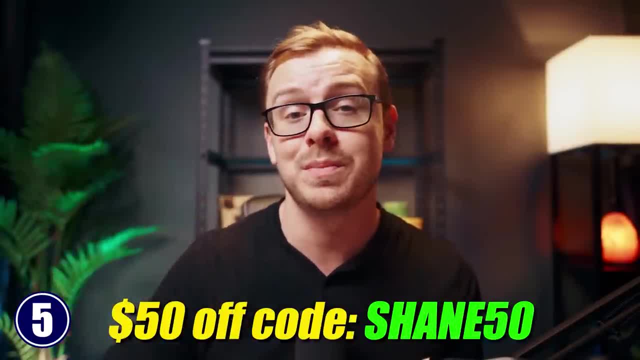 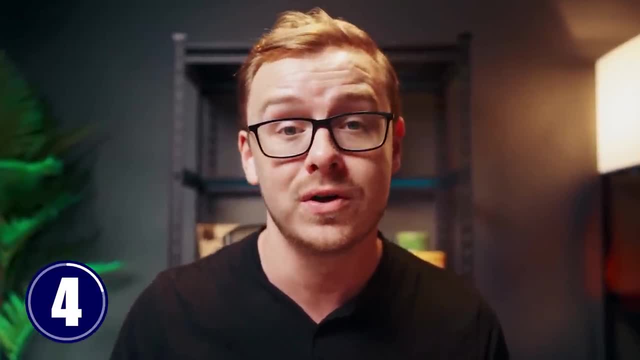 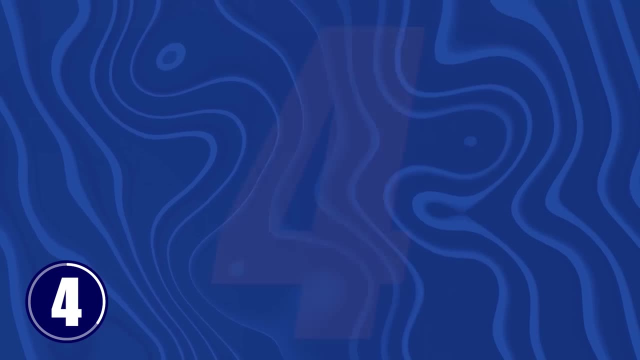 really good, But some of them are better than others, And software developers know the language of robots to command them what to do. But the people who give those robots life are going to be electrical engineers- And our entire society runs on electricity And electrical engineers. 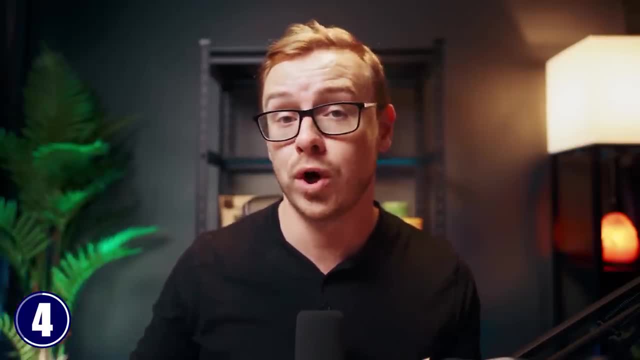 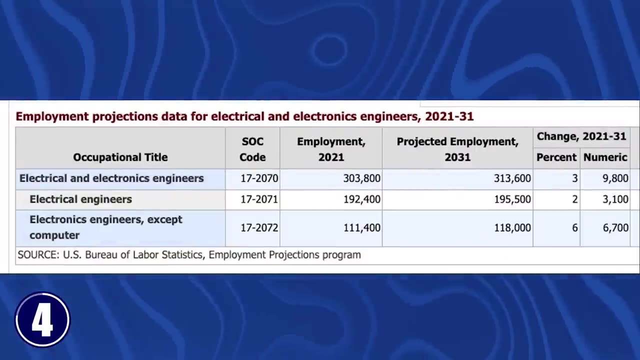 are the ones who design and build those systems that make everything work. Now, with this one, you'd expect to make about $88,000 a year in the entry level job And as an electrical engineer. it's only growing at about 2% over the next 10 years. But there is a ton. 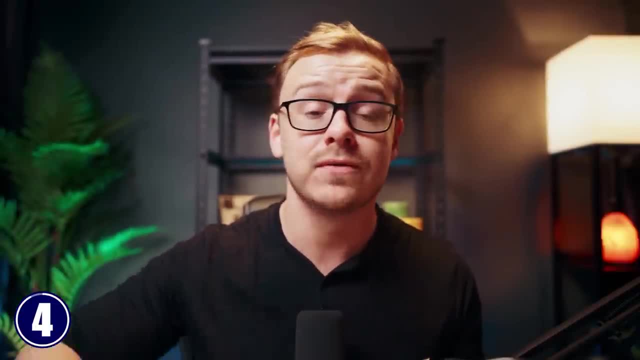 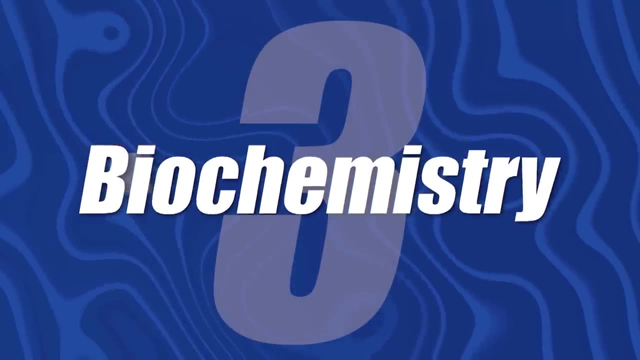 of different careers that you can go into, So this one is pretty rigorous. It's for people who love math and science, And they also aren't afraid of getting shocked. Now the next one on the list is going to be a science related degree, And everybody thinks that all STEM degrees are 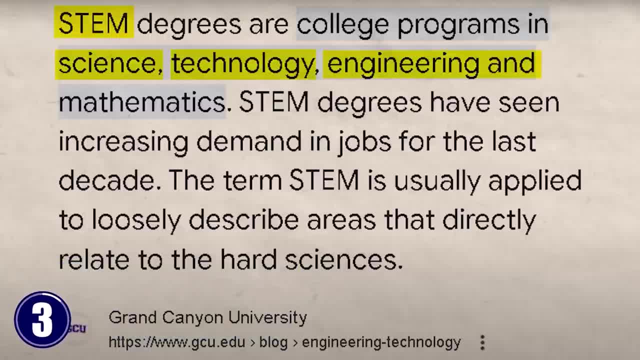 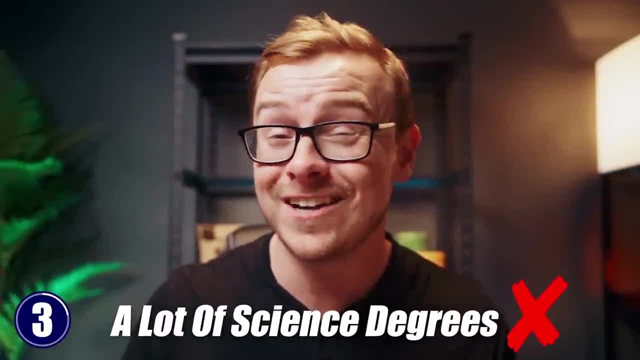 great, But the truth is STEM stands for science, technology, engineering and mathematics, And the last three, the TEM, are much better than science. A lot of science degrees are actually not good or in some case, they even fall into the category of being borderline, useless And, sadly, science. 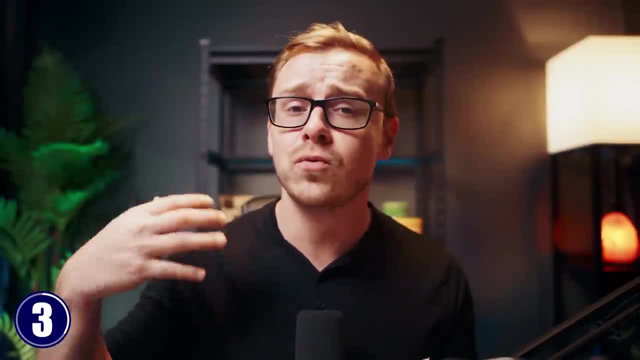 is a completely different field than science. It's a completely different field than science. It's a completely different field than science. It's a completely different field than science And for some reason, they seem to be really confused about basic biological principles, like people who 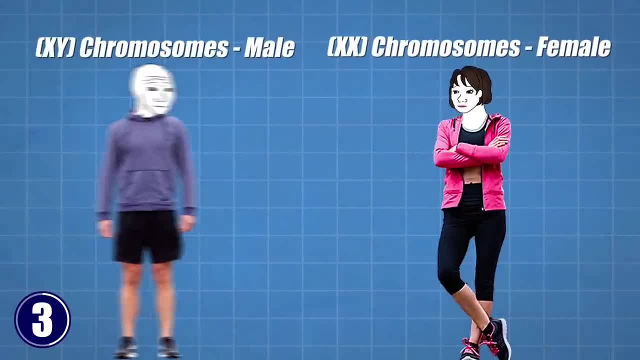 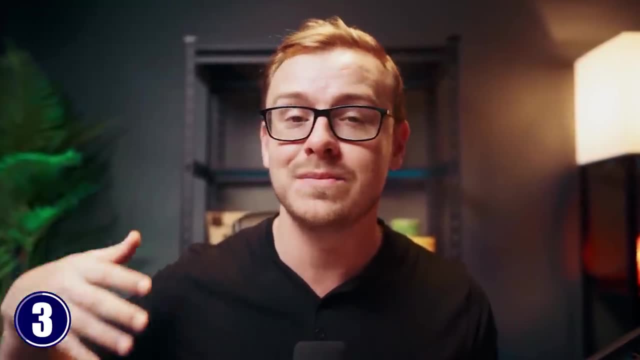 have XX chromosomes are women and people who have XY chromosomes are men, And they are literally letting men compete in women's sports right. I didn't think I would ever see this in my lifetime. This seems like some sort of like Salem witch trials type of thing. It seems like something. 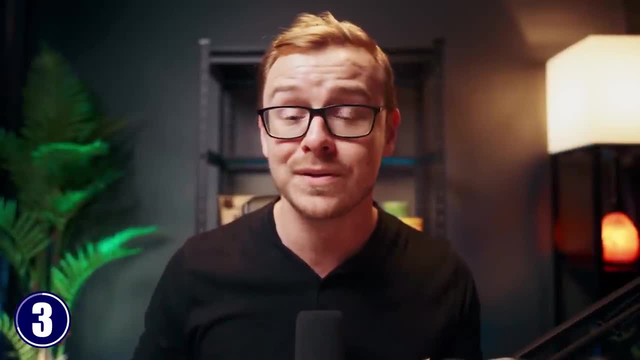 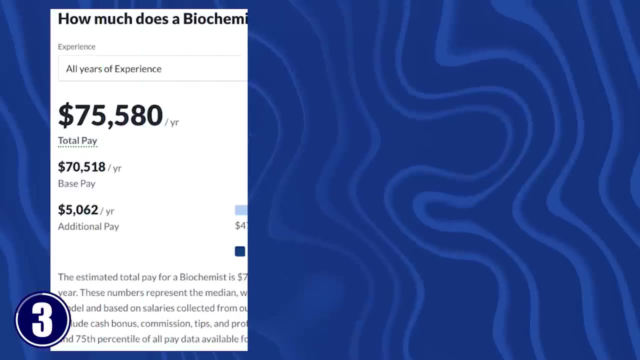 that you read about in history but you think, oh, this is never going to actually happen. But nope, it is actually happening right now. So unfortunately science- as much as I love, it- is a complete joke right now. Now, if you get a job as a biochemist, you can expect to make about 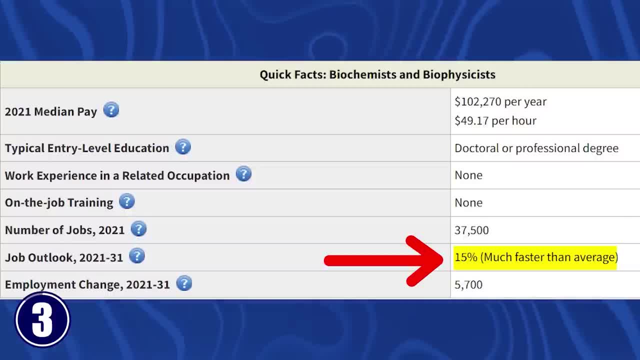 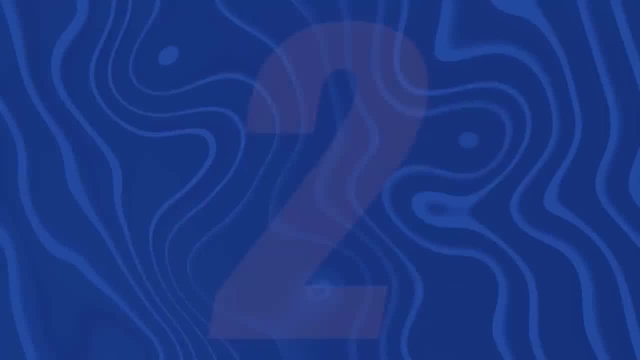 $75,000 a year, And this one is expected to grow at about 15% over the next 10 years. So biochemistry is one of the few science related degrees that are still really good. Now the next one on the list. 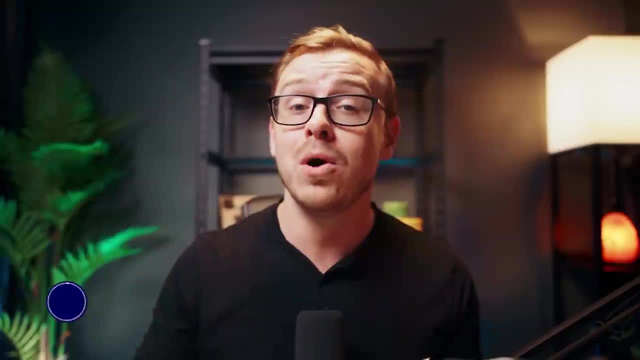 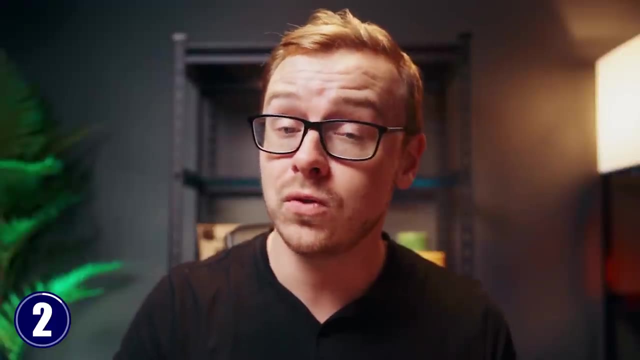 is going to be a social sciences degree And, yes, most of these types of degrees are not very good when it comes to the numbers. However, I think a lot of them are extremely interesting, And one of the most interesting ones is actually still a pretty good degree to get, And this is going to 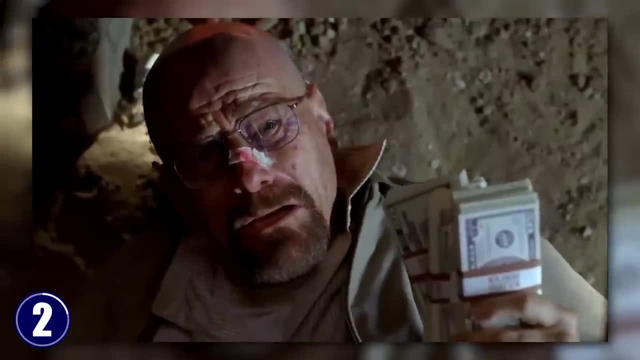 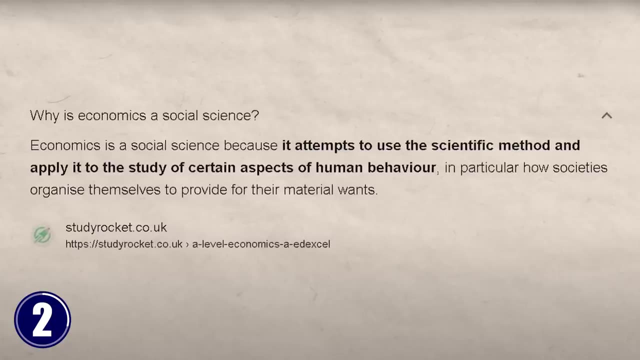 be studying how people make money, spend money and stress about money, And a lot of the time it's going to be done from a big picture perspective. Now, what's so interesting about economics is, yes, there is a logical kind of like science, fact based component to it, But at the same time, 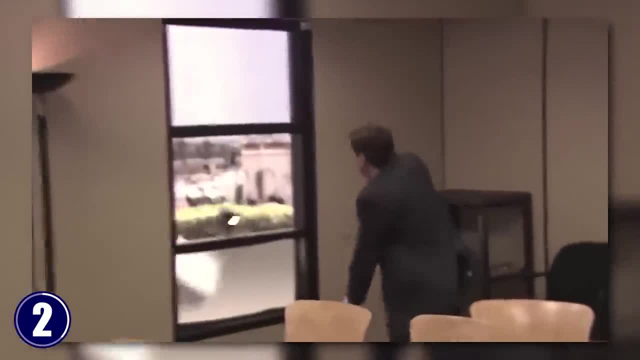 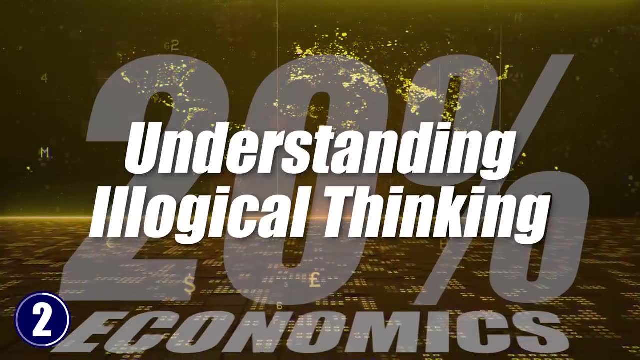 you're still dealing with human beings, and people are extremely illogical. So 80% of it is kind of like science, math, analytical thinking, but 20% of it is just understanding illogical thinking, And there's definitely a part of economics that has sort of been hijacked as well. 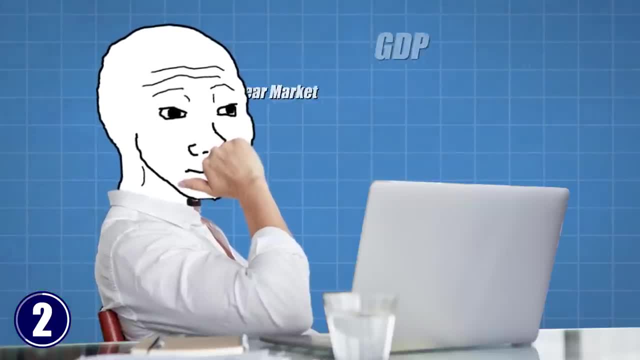 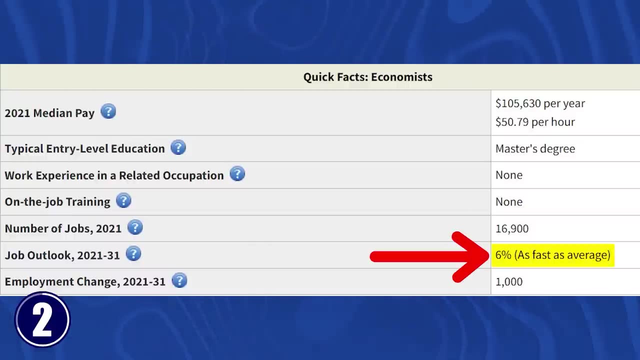 where basically, it's just a bunch of fancy words and terminology to make up excuses to make the money printer go burr. Now economists make about $99,000 a year and it's expected to grow at about 6% over the next 10. 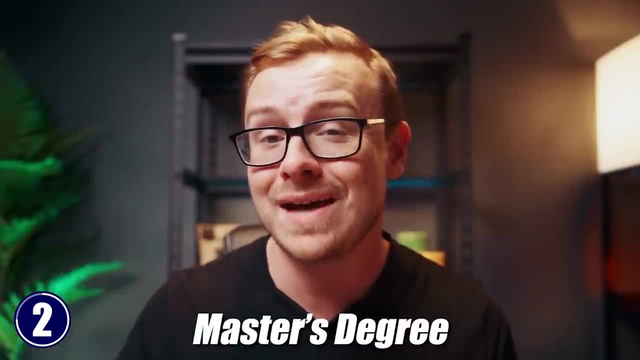 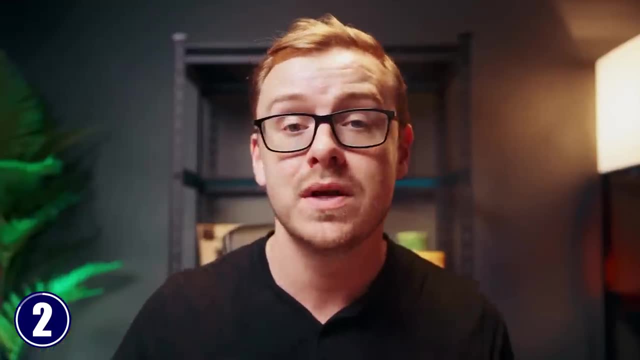 years. But keep in mind, to become an economist, you typically have to get a master's or a doctorate. With that being said, there's a lot of jobs out there where it does not require a master's or a doctorate and you can get into it with just a bachelor's, So this one is great for. 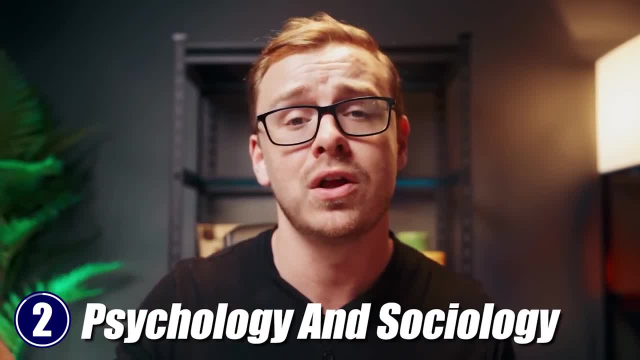 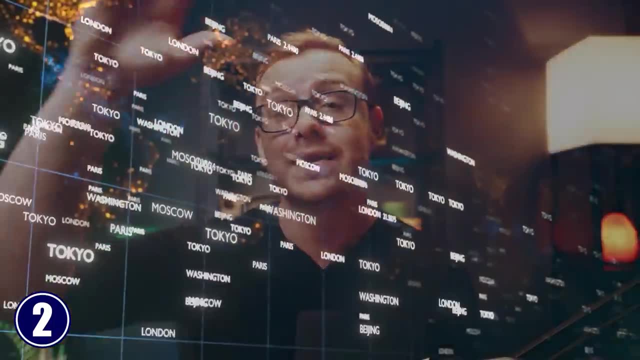 people who sort of like money, but they also like psychology and sociology at the same time, And you can kind of understand why human beings do what they do when it comes to money, And it also helps you understand how the entire world works as well. Now the next one I'm going to talk. 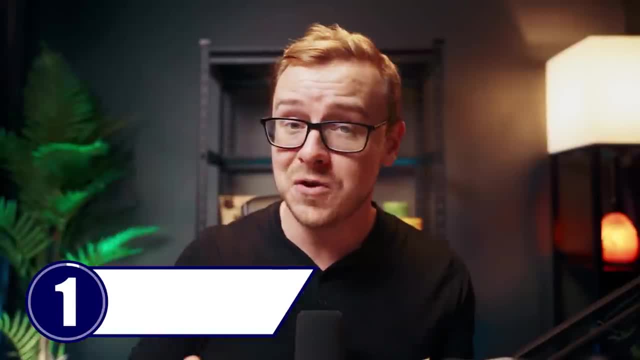 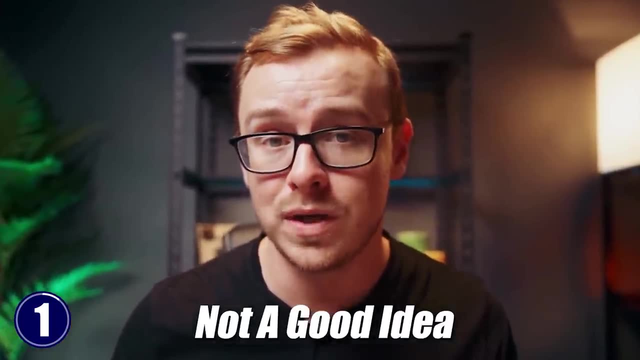 about is going to be an art-related degree. And I have to admit something: I sort of tricked you because I'm going to tell you right now: 99% of the time it's not a good idea to get an art-related degree. So I'll go ahead and give you an example of where it would be a good idea. 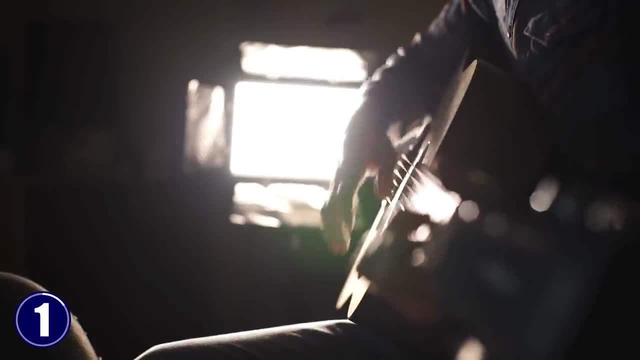 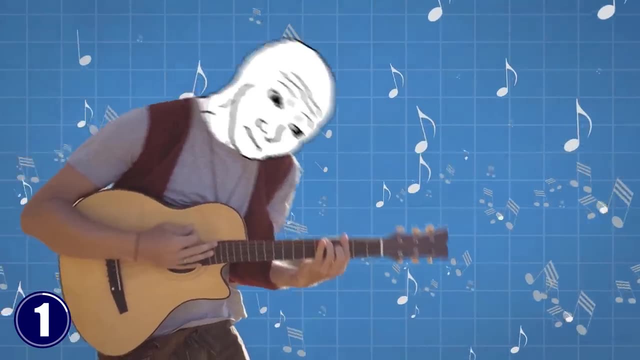 If you are a world-class classical guitarist, for instance, right, And you're like in the top 99.9th percentile and you're trying to get into the top 99.99th percentile and you have an opportunity to go to a top level school where you're going to get to work with people who are 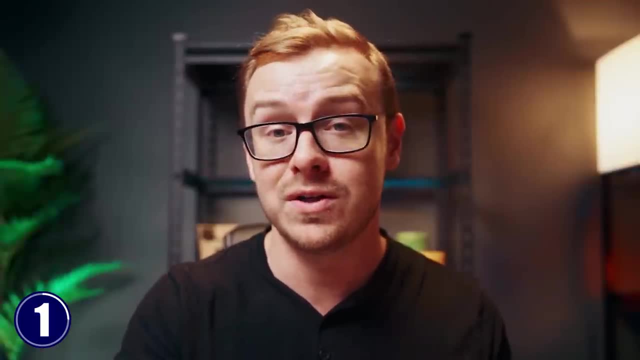 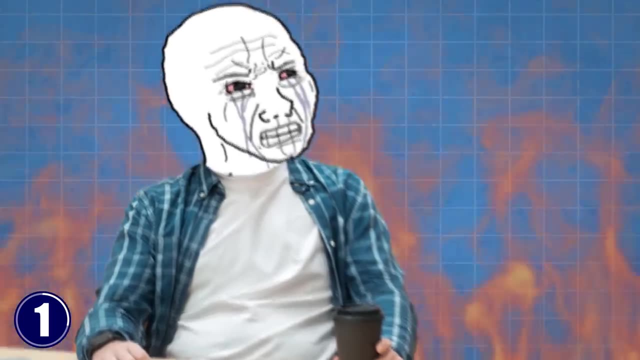 even better than you, then it might be a good idea to get an art degree, But in almost every other case it's not a good idea, And the reason for that is because universities are never going to be able to teach you what is up to date in art, And it's going to cost you a lot of money. 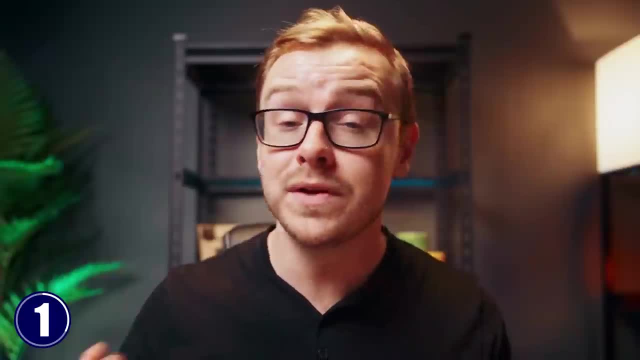 and it's probably going to set you back when it comes to you reaching your goals. Now, this is coming from somebody who's technically an artist. I mean, I guess I'm an artist because I make YouTube videos, As cringe as that sounds. 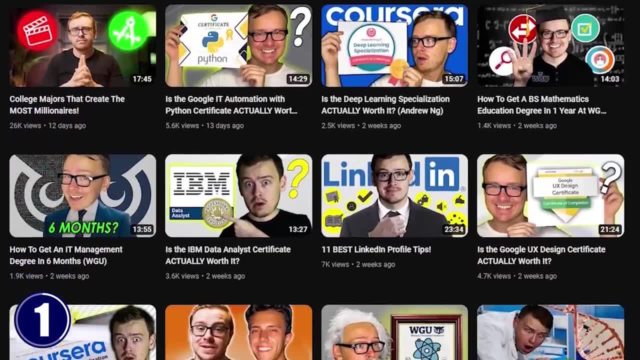 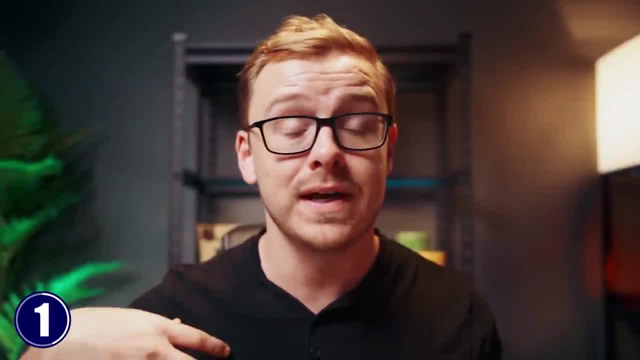 I mean, I make some really good modern art when it comes to my thumbnails, for instance. I think my O-face on thumbnails is as good as anybody else out there, And I have absolutely no problem with artists. In fact, I would say the majority of my friends are artists. But what I would recommend 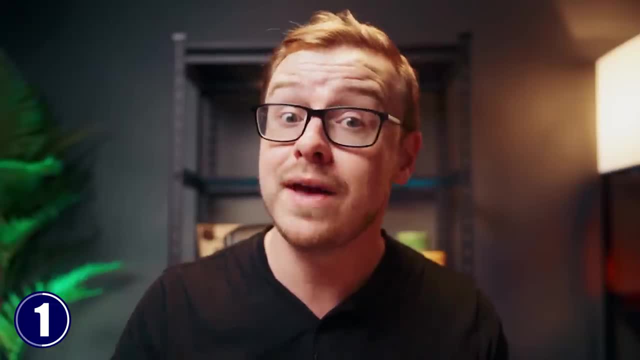 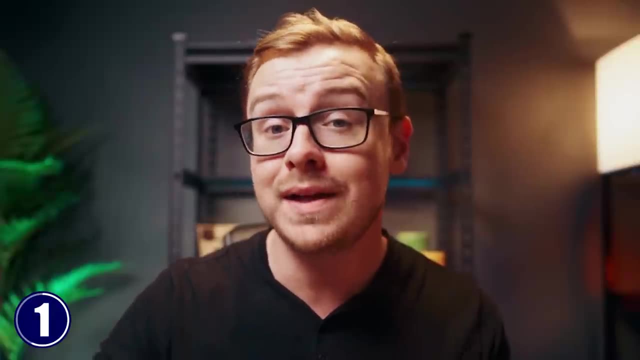 if you want to actually make money for a living from your art- which, by the way, you don't have to do. You can just keep it as a hobby, And in that case you'll probably end up enjoying it more. But if you do want to make money, actually get a job, from your art, I highly recommend reading.